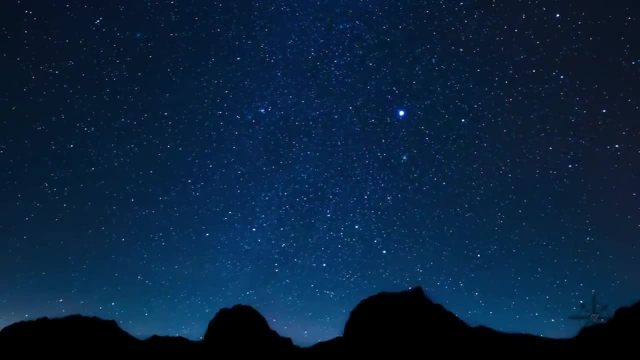 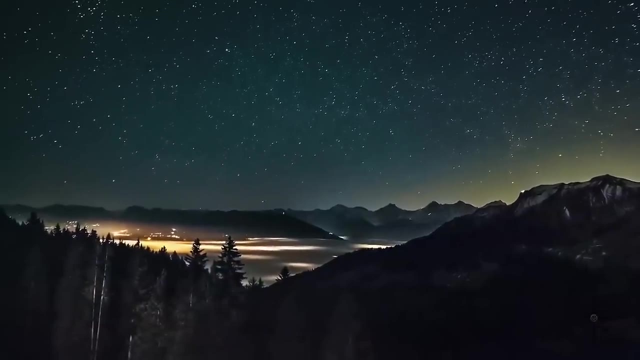 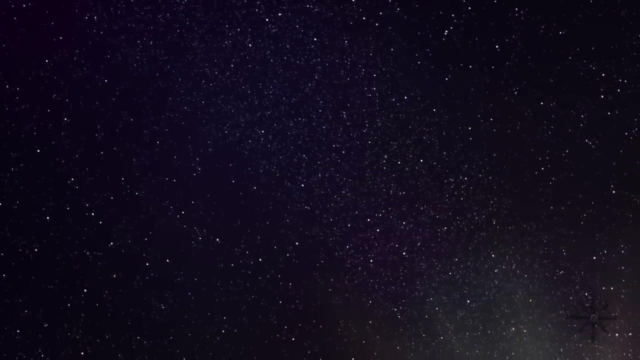 Without clouds, about 6,000 stars are visible in the night sky from anywhere on earth. This number is lower in areas of heavy light pollution, but for the most of human history this is what we had to look up to. In earlier times, there were many ideas as to what the stars were. The Greeks 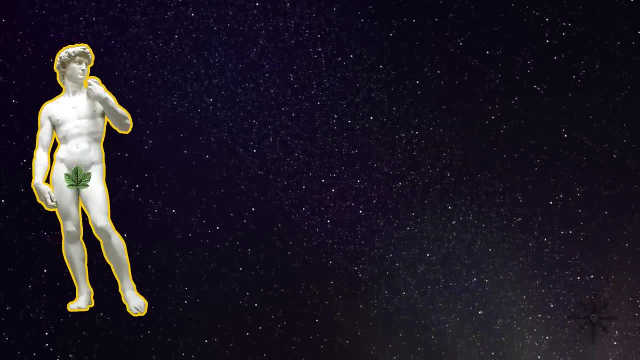 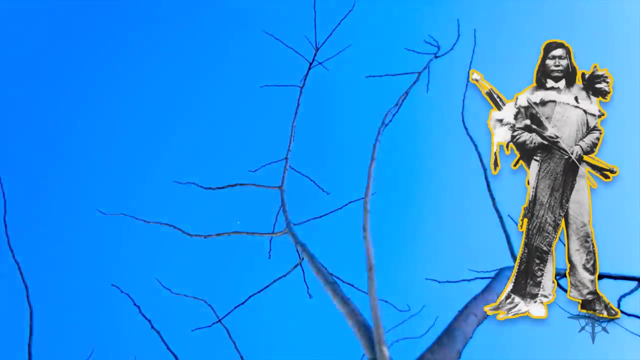 saw constellations who were sentient divine beings awarded with a place among the stars for some great deed done long ago To the Paiute tribe, who lived in the Great Basin of North America. stars were the children of the father-son and the mother-moon, eaten every day by the light. 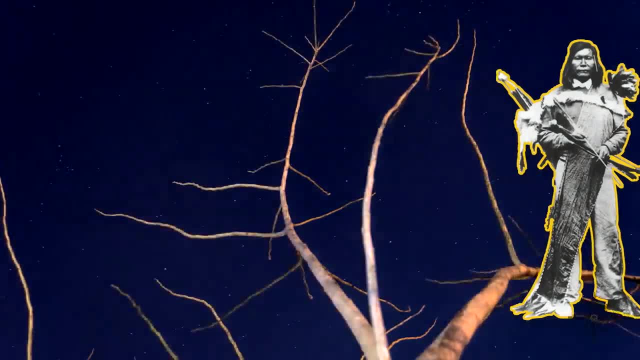 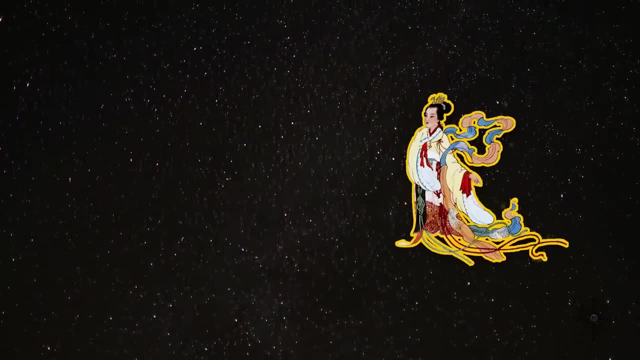 of the sun and nursed back to life by the love of the moon. In Chinese mythology, some stars represented actual people. One is Zhi Nu, the girl who weaves the clouds, and another is Niu Leng, the herdsman who cares for the cattle of the heavens. The two were in love, so the gods 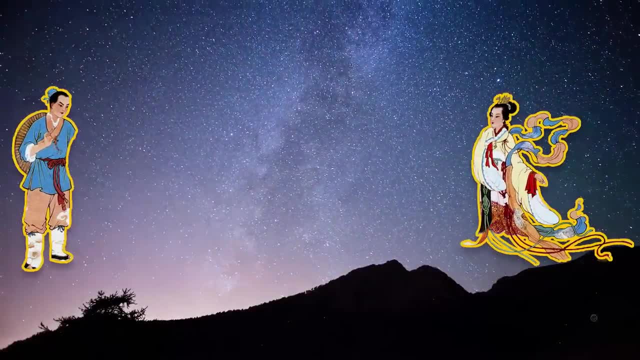 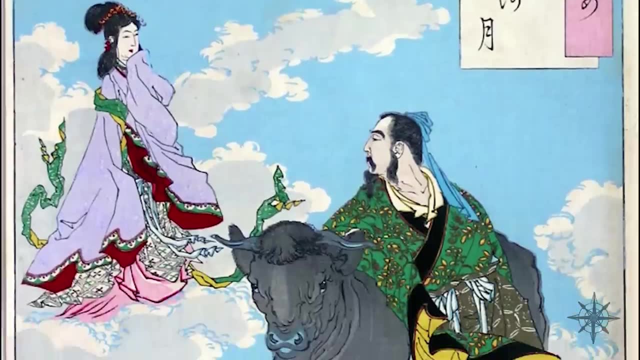 placed them on either side of the Milky Way to make sure they were never distracted from their duties. Only once a year, on the seventh day of the seventh month, the two loved ones were allowed to meet, when the birds in the sky will form a bridge across the Milky Way To the Yakut. 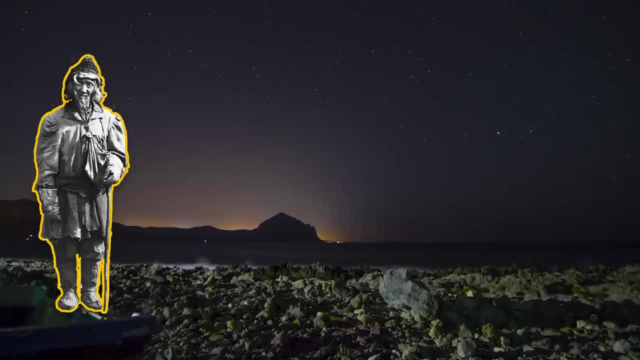 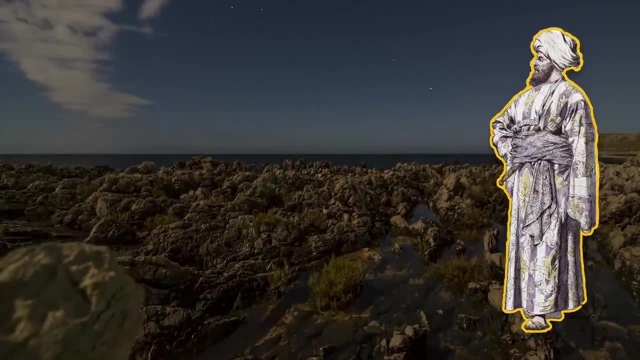 tribe of Siberia, the stars are crystal lenses used by the gods to watch the earth, And for the Turk people of Central Asia, the sky was one big tent and the stars were nothing more than small rips in it. Of course, we know now that all these stories are wrong and in fact stars are giant. 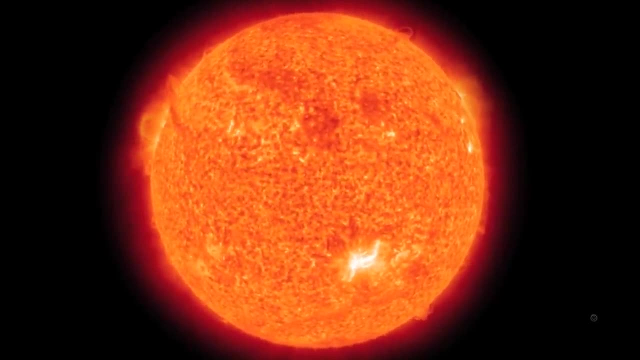 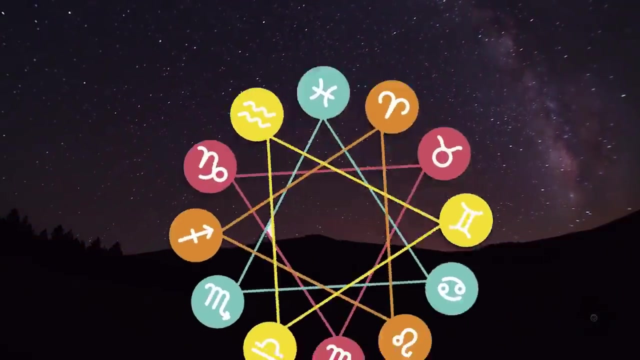 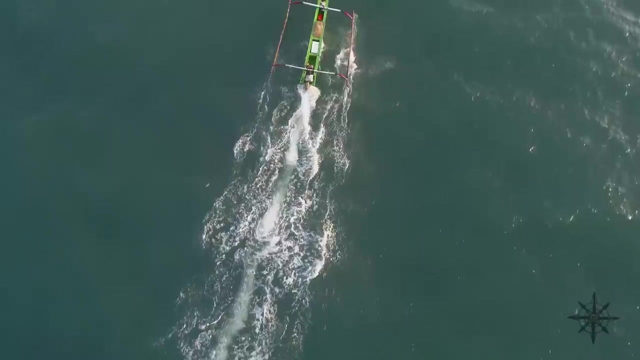 gas clouds glowing from the process of nuclear fusion billions of miles away. But of these ancient understandings of the stars, one remains true to this day. No, it isn't zodiac readings, but navigation. Ancient travelers and modern sailors and pilots alike would use the stars to voyage through their lands and to discover new ones. So how? 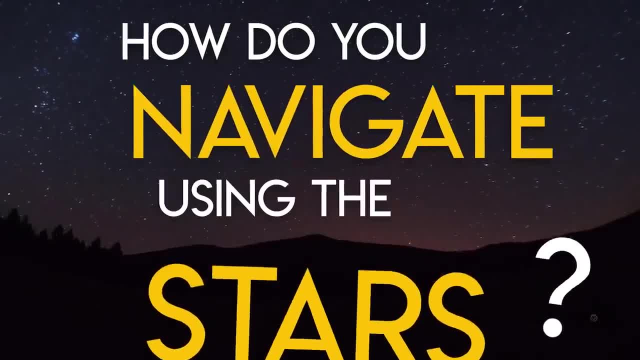 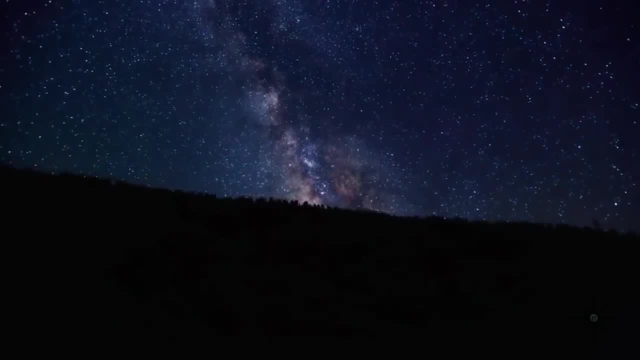 did they do it? How do you navigate using the stars? Well, first, a quick look at some time-lapse photography will show that the stars are not static in our skies, but instead they streak across the sky as the earth revolves. Using a moving star as a reference point is 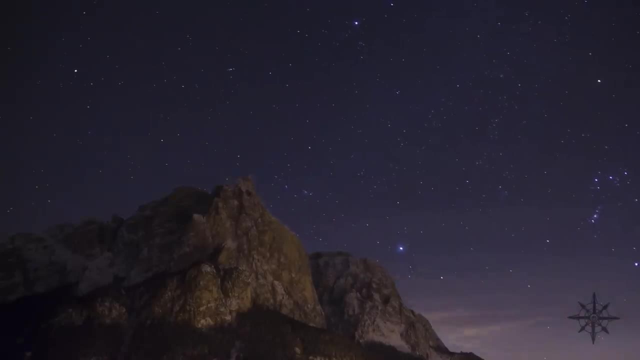 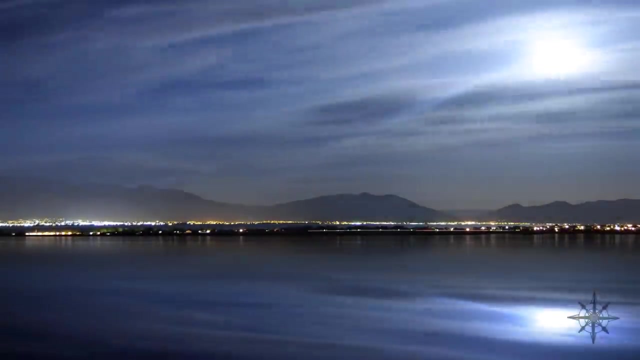 problematic, especially for long journeys, so you can't just pick any star in the sky and follow in its direction. Another problem is present for the sun and moon for navigation, as they will move across the sky in a similar way And while many think they may be able to use the sun at the very. 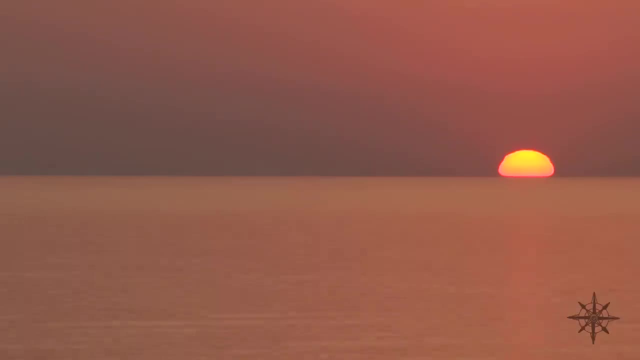 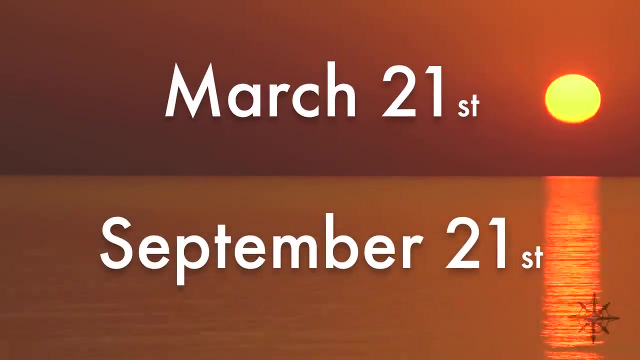 least to rise in the east and set in the west. due to the earth's seasonal tilts, it's rare that the sun ever rises in true east or sets in true west. Only on the equinoxes at the equator does this occur, just twice a year. So what's needed is a reference point. 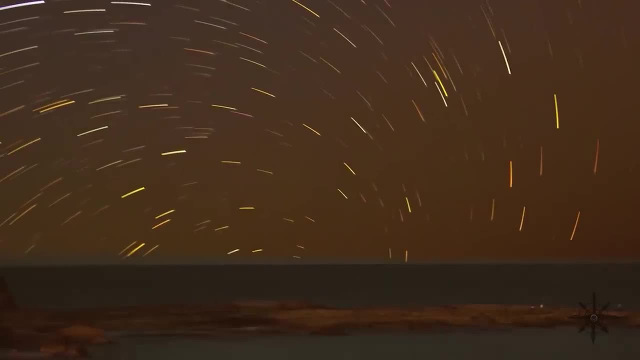 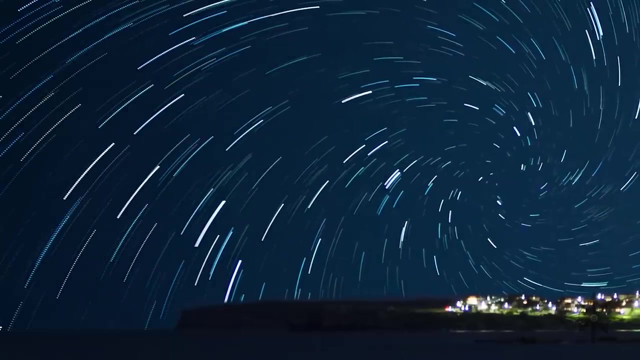 that, no matter the year, month, week or day will always lead you in the same direction. One last thing before we get started is the stars used for navigation vary depending on which hemisphere you're in- north or south, as the stars in the northern hemisphere can't be seen from the southern hemisphere and the 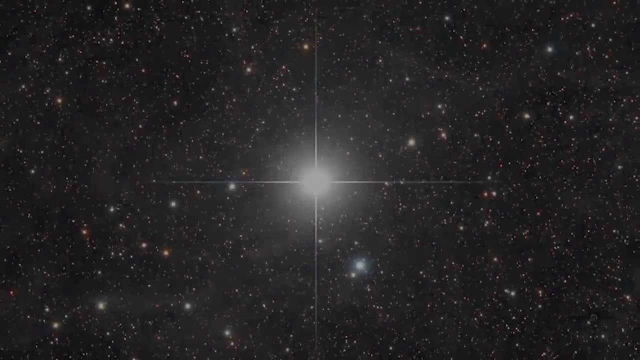 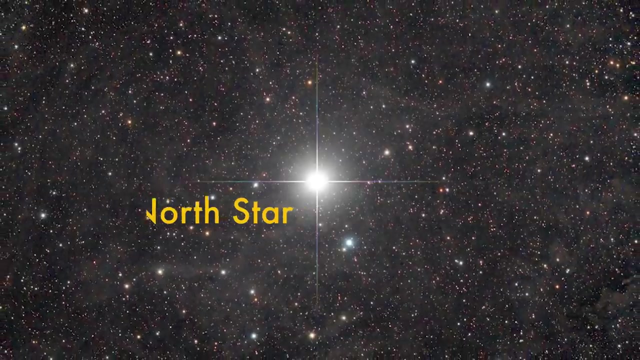 other way around. So, knowing that, let's get into it. First, we'll start in the northern hemisphere, and here we'll find perhaps the most well-known star for navigation, Polaris, the north star. By random chance, Polaris sits virtually on top of true north, just a fraction of a degree. 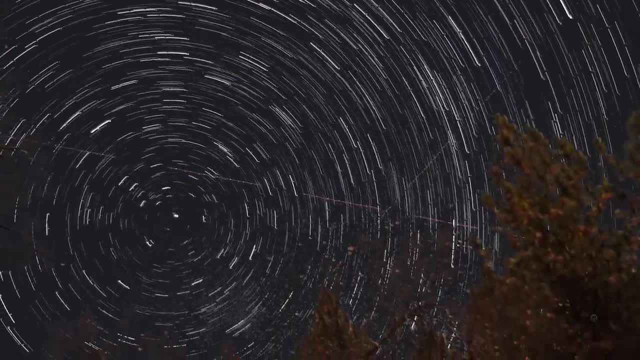 off and because of this it barely moves in the sky, while all the other stars spin around it. This can be seen by the fact that Polaris is the northern hemisphere and the stars seen best in long exposure photographs, where all the moving stars make long streaks through. 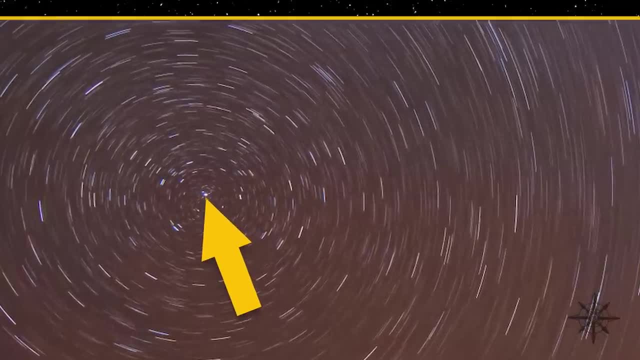 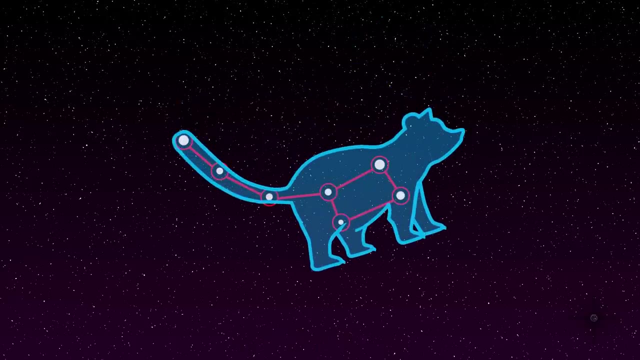 the sky, but at the center is Polaris, hardly moved at all. Finding the north star is fairly simple too. It's the brightest star in the constellation. Ursa Minor, the little dipper or the little bear- Yeah, I don't see it either. 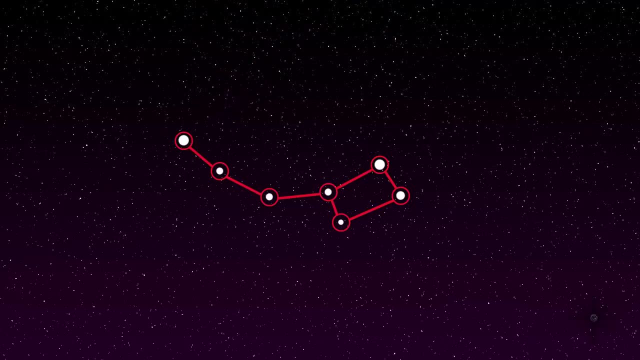 Polaris is the last star in the handle. If you're having trouble spotting it, you can look for Ursa Major, the big dipper, or the big bear, which I find much easier to spot. Once you've found the big dipper, you can use its end stars called the Dubhe and Merak. 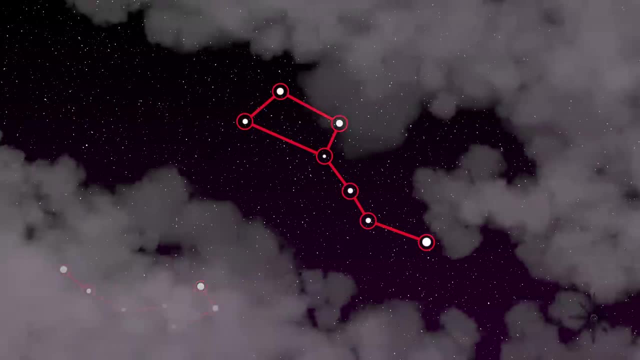 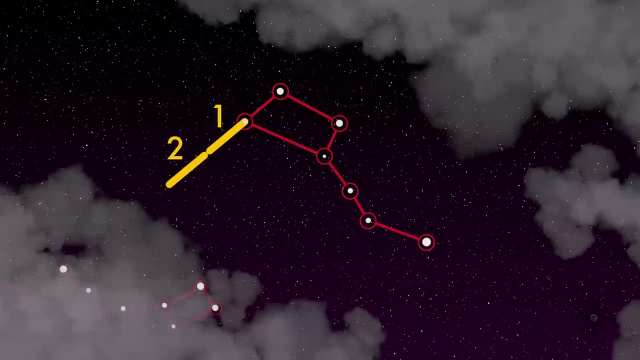 to follow the path they make straight to Polaris, If clouds are covering Polaris but not the big dipper. know that Polaris lies roughly five lengths of the distance between Dubhe and Merak away. Also, be aware that while Polaris stays relatively still, the 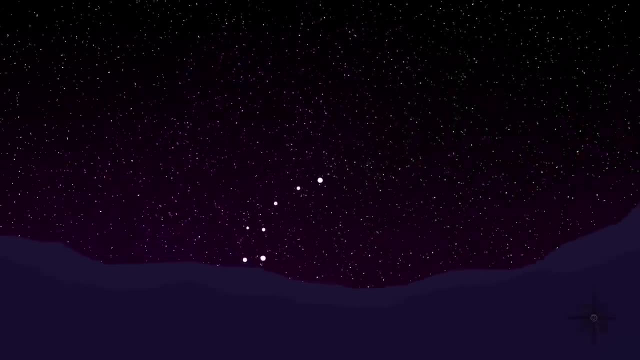 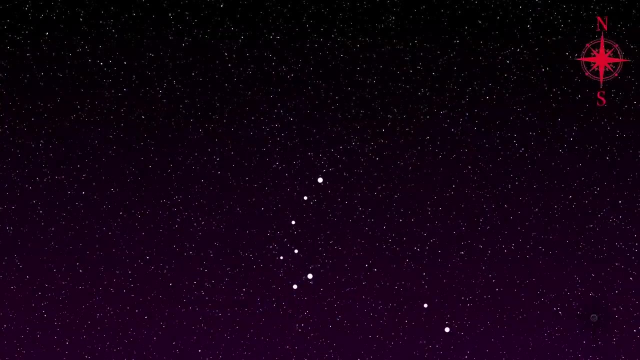 big dipper, like the rest of the stars, will move and sometimes may be covered by objects on the horizon like mountains or trees. so it's best to look for Polaris on high ground. Okay, so what about if we're going south? Can we just find the north star and sail in? 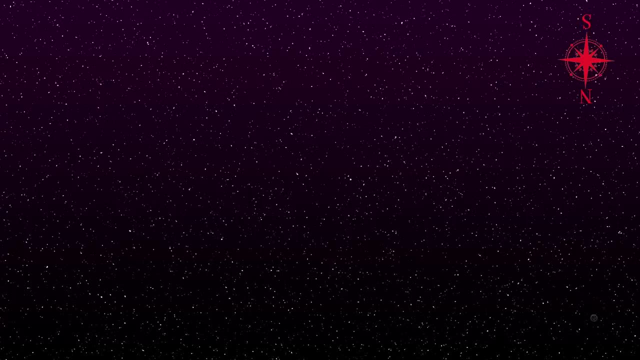 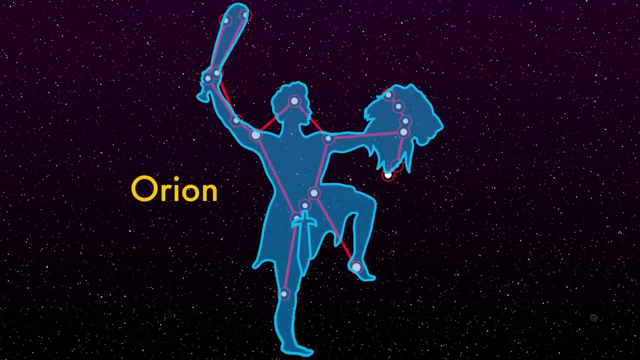 the opposite direction. Well no, Without a point to aim your ship at, there's no real need to ensure you're sailing in the right direction. Instead, you'll need to find another well-known constellation, Orion. And if that just looks like a bunch of random stars, don't. 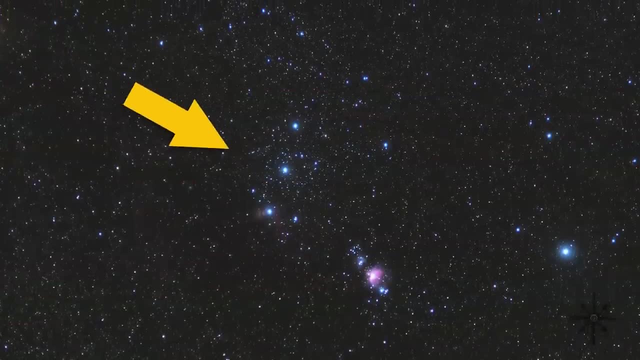 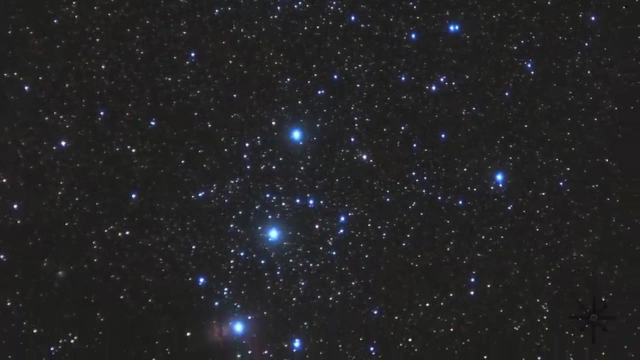 worry. All you need to know is his belt. These three close stars in a straight line: Alnitak, Alnilam and Mintaka. Mintaka comes up again later, so try to remember it, But from here you'll need to find what's called Orion's sword, which hangs from his belt. It's these: 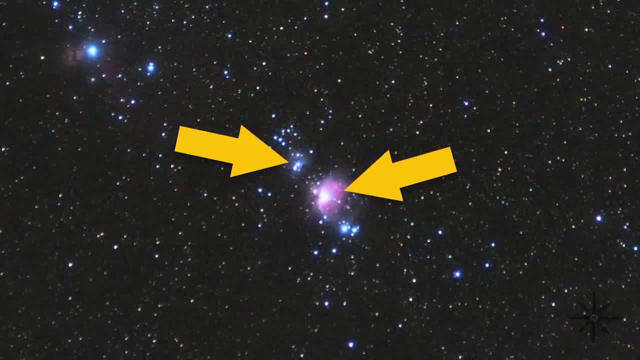 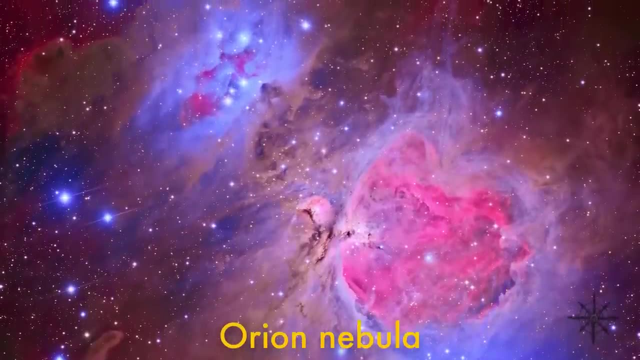 three stars here, made from a dim star, a fuzzy star and a bright star. That fuzzy star isn't actually a star, but a huge gap in the sky. There's a gas cloud called the Orion Nebula where new stars are actually being made, If 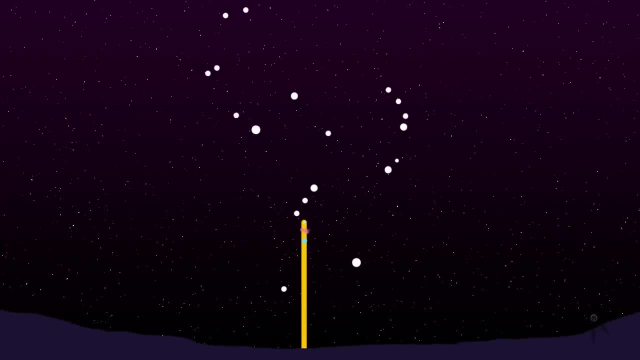 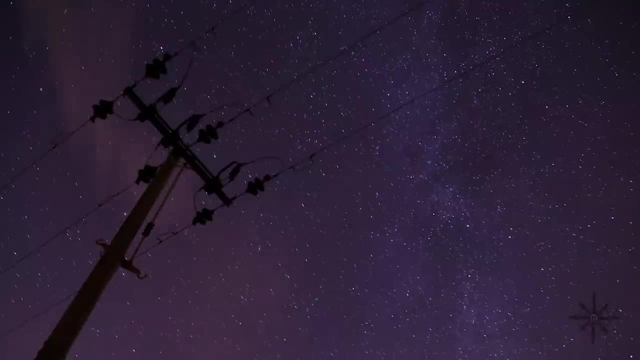 you follow the direction of this sword down to the horizon, this point should lead south. This gets a little inaccurate when the constellation is lower in the sky, but should still bring you south. Okay, now we're in the southern hemisphere, and this is where things start getting a little. 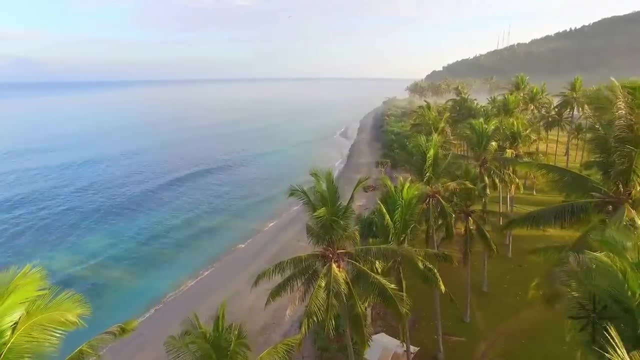 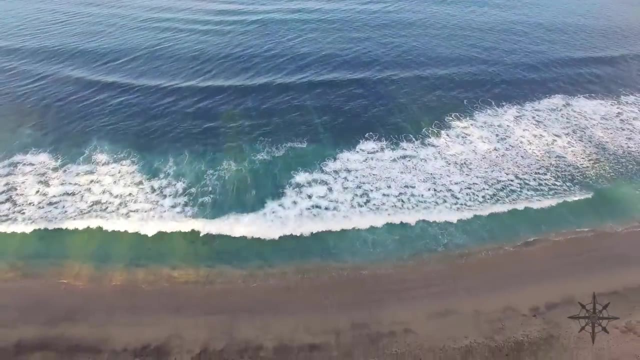 tough, But considering most of the Earth's oceans are in the southern hemisphere, it's still very much worth learning. Here we'll find probably the second most popular method of using stars for directions, right after Polaris. If you're Australian, Kiwi, Papua New Guinean, Brazilian or Samoan, you're likely familiar. 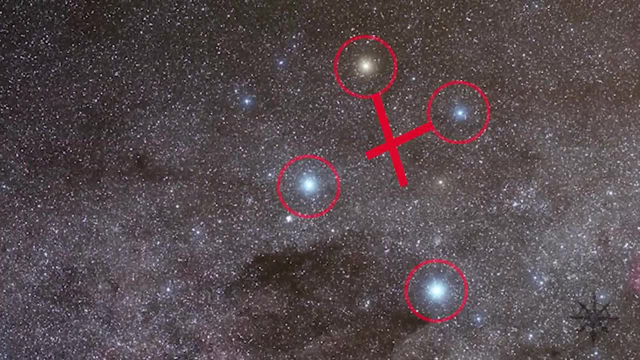 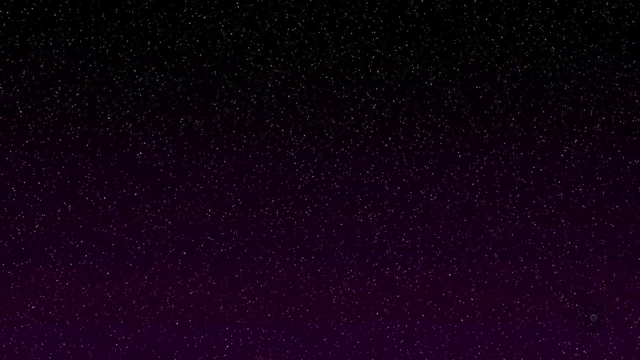 with it already, And that's the Southern Cross, more officially known as Crux. It can be seen as a cross with an extra blemish star right here. Some may find this one a bit harder to find in the sky, as just about any four stars can make a cross in the sky, But there's. 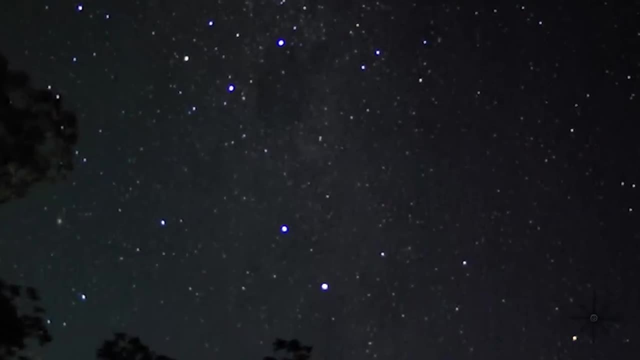 a way to help you find the right one. To the side of the Crux, there will always be two bright stars, sometimes easier to spot than the Crux itself. These are called the Pointer Stars, and you'll need them again later. The Pointer Stars are the stars that you'll need. 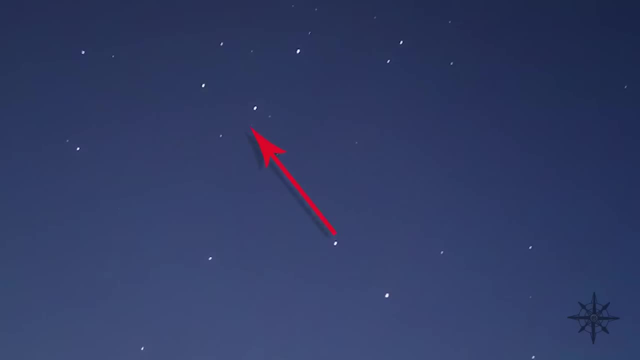 to make a cross in the sky. The Pointer Stars are the stars that you'll need to make a cross in the sky. The Pointer Stars always point towards the Crux and can confirm for you, if you're sure, that you are in fact using the proper stars. 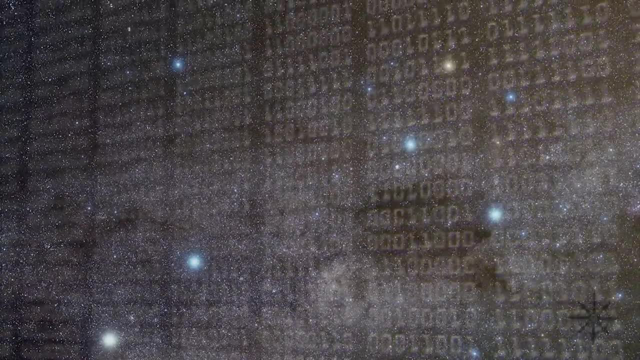 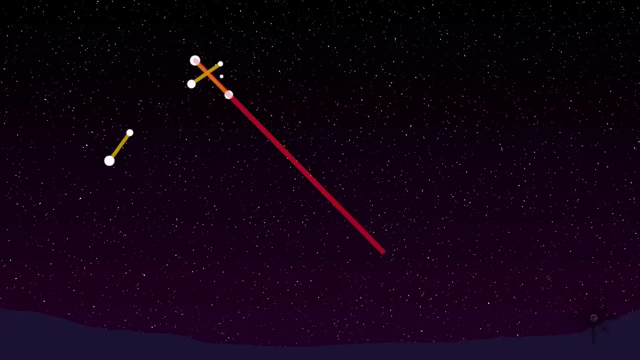 After you've located the Crux and its pointers, you're going to need to do some more line drawing in your head. Say, your sky looks like this. Using the top and bottom stars of the Crux, draw a line out from the bottom of the cross, Then from the two Pointer Stars, draw.